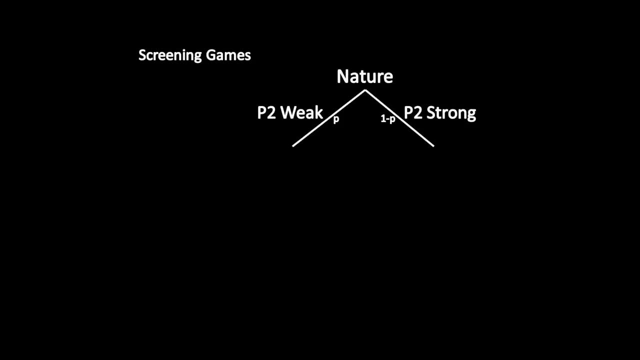 So let's get to it. Let's see a game of incomplete information. Games of incomplete information tend to start out in the same way. It's a move by nature. Nature is an autonomous actor. It's not strategic. it behaves randomly in a way that's defined. 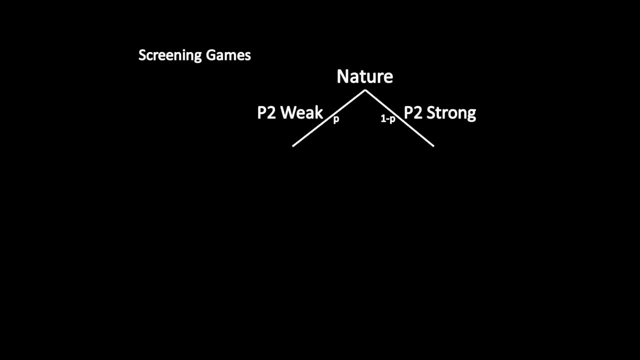 by the parameters of the game Here. nature is either choosing player 2 to be weak or player 2 to be strong, And specifically it's going to choose weak with probability p and strong with probability 1-p. p and 1-p are the prior. 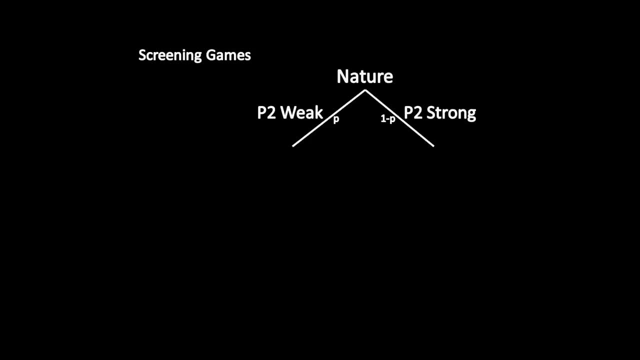 beliefs that player 1 is going to have about player 2's type. So if we flesh out the rest of this game, it's country 1 and country 2. in some sort of crisis over a good that they both want, Player 1 can either escalate the dispute or 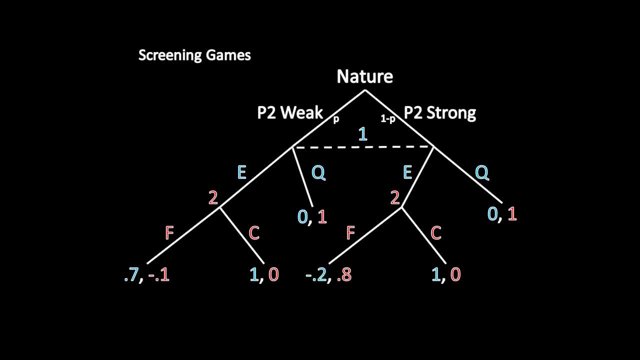 quit, And if player 1 escalates, then player 2 can either fight over the good or concede. You'll notice that after nature makes its move, we have a dashed line connecting player 1's choices. This is reflecting the fact that player 1 is in the dark. He doesn't know whether player 2 is weak. 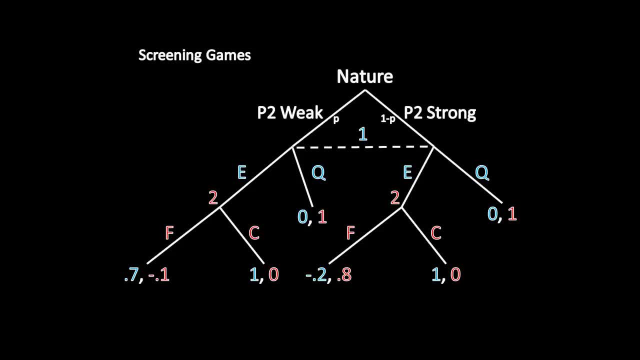 or strong. he just has that prior belief of p and 1-p over those two different outcomes. In contrast, player 2 has complete information. Only player 1 has incomplete information. Player 2 knows whether she's weak or she's strong, so there is no corresponding dashed line. 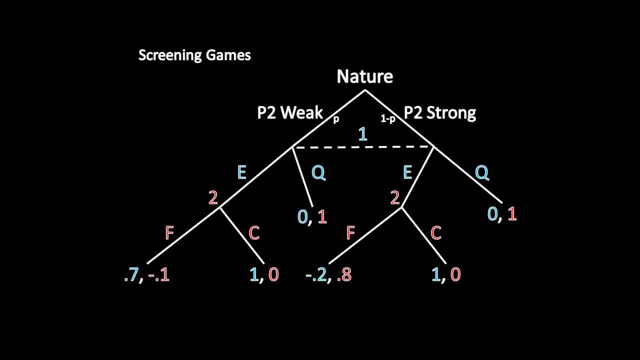 To fill out the rest of the payoffs here if player 1 quits. it doesn't matter whether player 2 was weak or strong. player 2 is going to capture the entire good and get a payoff of 1, whereas player 1 is going to receive nothing at all. 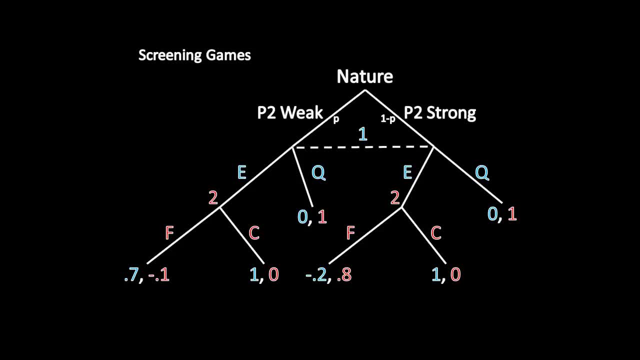 If player 1 escalates now player 2 has to make a move. She'll either fight or concede. If she concedes once again, payoffs are not a function of what nature drew earlier. Player 1 will capture the entire good for himself and player 2 will receive a payoff of 0.. The types matter. 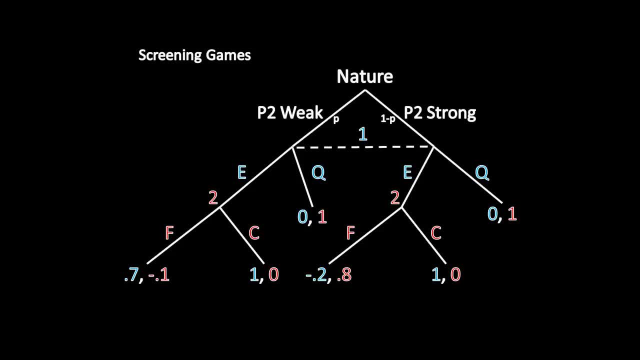 if player 2 fights. If player 2 is weak and fights, then we're on the very left edge of the game tree and player 1 will receive a payoff of 0.7.. He's doing very well for himself in this war. 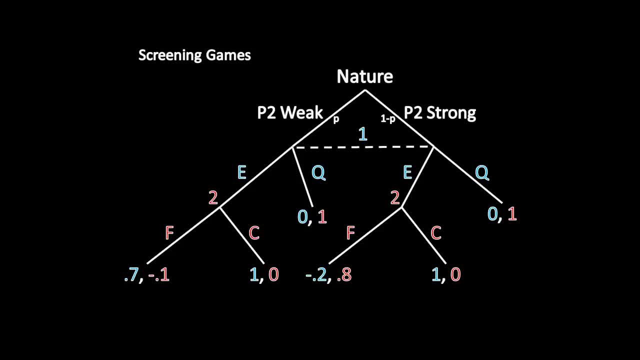 because player 2 is weak, whereas player 2 is suffering quite a bit. She's receiving a payoff of negative 0.1. The reverse is going to be true if player 2 is strong, If player 2 is strong and she fights well, now player 1 is getting a negative payoff- negative 0.2, and player 2 is going to be. 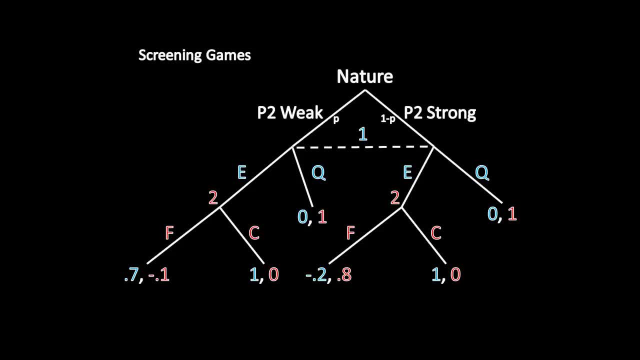 doing quite well for herself, She's getting a payoff of 0.8.. So this is the game. Let's go ahead and solve this and let's see why screening games- situations where the uninformed actor is moving first- is easier to solve, for Let's see why that's the case. Well, think about what player 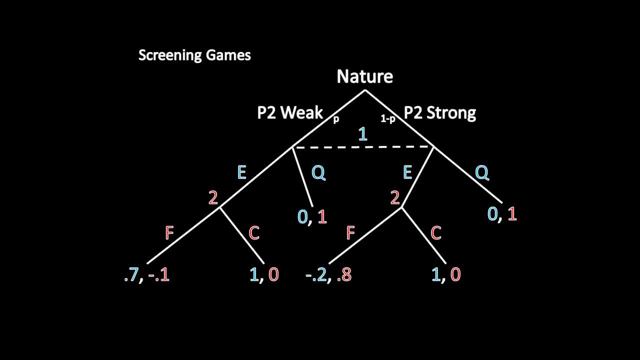 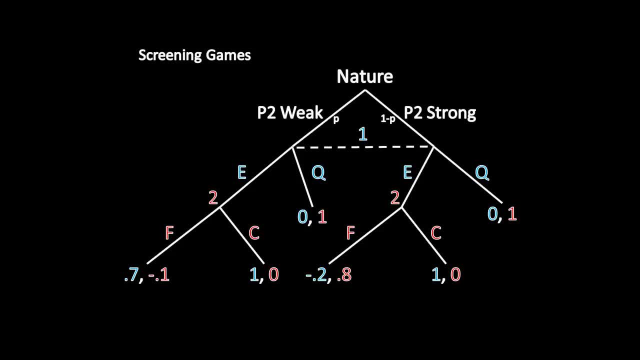 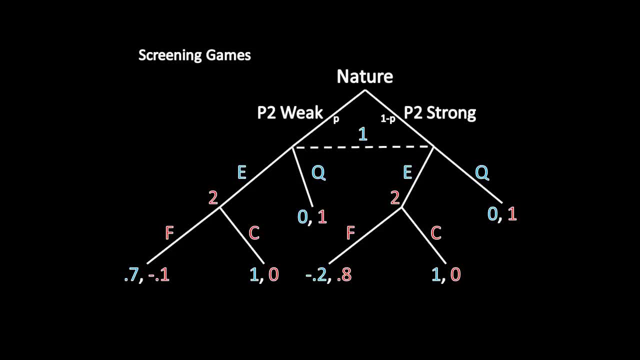 bigger. Essentially, all player 2 has to do is apply backward induction, just like what we would do for complete information games. So let's look at the weak side. If player 2 fights, she receives a payoff of negative 0.1.. If she concedes, she receives a payoff of 0.0.. 0 is better than a payoff. 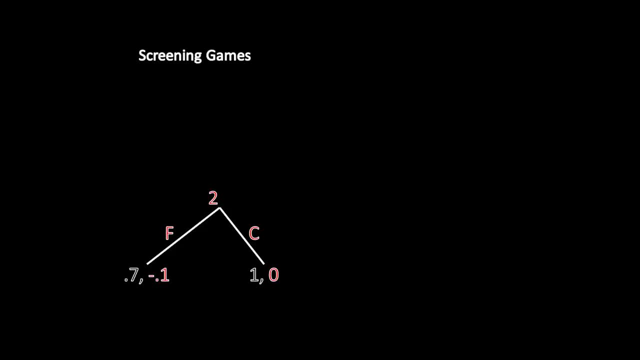 of negative 0.1, so she should concede, and she should concede, and she should concede, and she should concede. in this case, What about on the other side? Well, if she fights, she gets a payoff of 0.8. here, If she concedes, she gets a payoff of 0.0.. 0.8 is larger than 0, so she should fight. 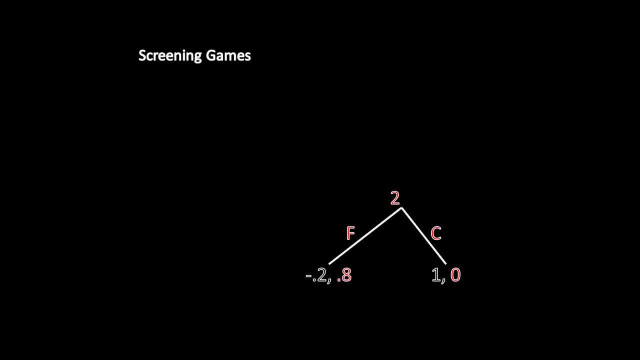 So that allows us to simplify the game tree again, just as we would in a game of complete information. So weak type is going to concede if player 1 escalates and the strong type will fight. Thinking about player 1's strategy is a little bit more complicated. 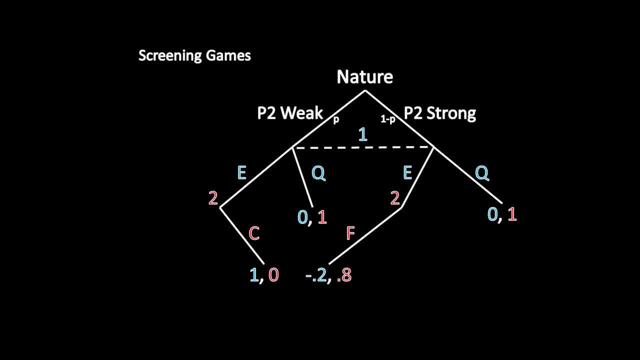 Now player 1 has to think about what's going to happen in the future if he escalates. and he doesn't actually know for sure whether player 2 is going to concede or fight. He just has a prior belief, and that prior belief is going to be enough to allow him to figure out. 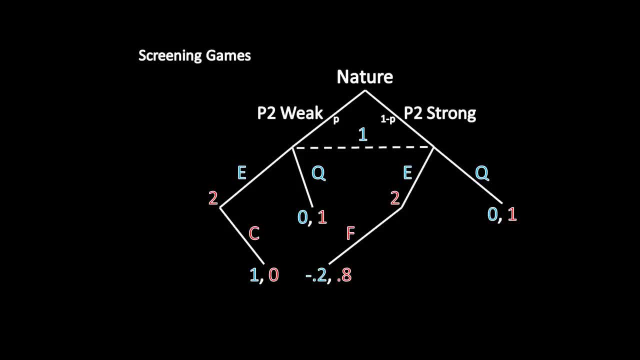 exactly what he should do. But there's actually something simpler we can calculate. first, We need to compare his payoff for escalation versus his payoff for quitting, and his payoff for quitting is very straightforward. It doesn't matter what player 2's type is, If she's weak or 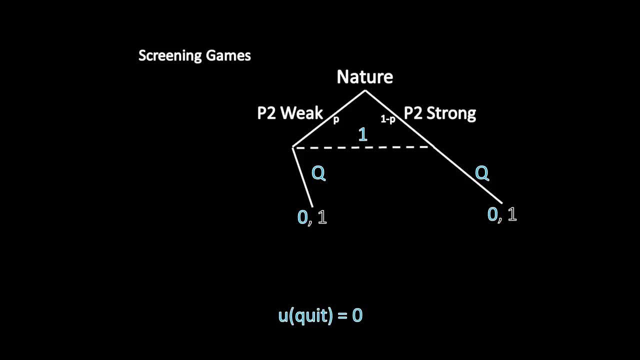 she's strong, player 1 is still going to receive a payoff of 0.0.. It doesn't matter whether player 1 is going to be facing a weak type or a strong type of player 2. in that case, However, if player 1 chooses to escalate, now the types matter, But it's still relatively. 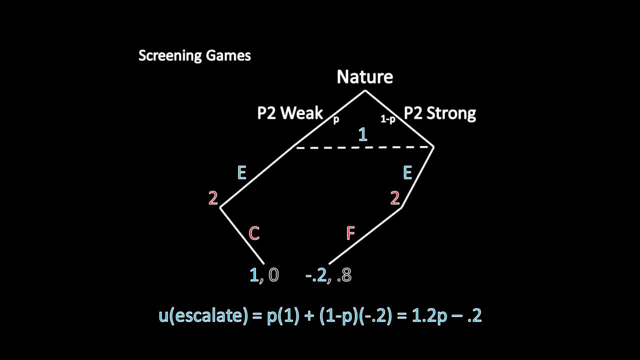 easy for player 1 to figure out what he should do and we can get that by calculating the payoff for escalation. If player 1 escalates, then with probability p, player 2 will get a payoff of 0.0.. In that case, player 2 will actually be a weak type and choose to concede. In that case, 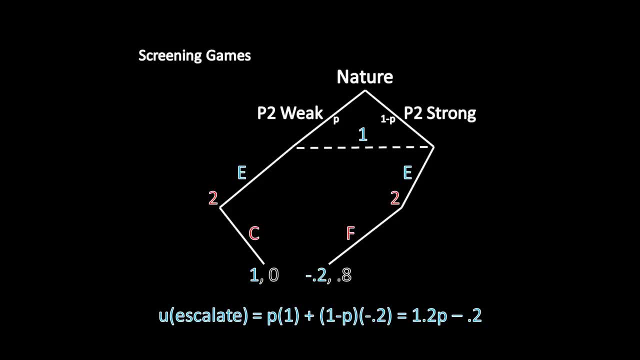 he gets a payoff of 1.. With probability 1 minus p, player 2 is going to be a strong type who will choose to fight him. He'll get a payoff of negative 0.2 in that case. So we can calculate those, sum them together and we get an expected payoff. 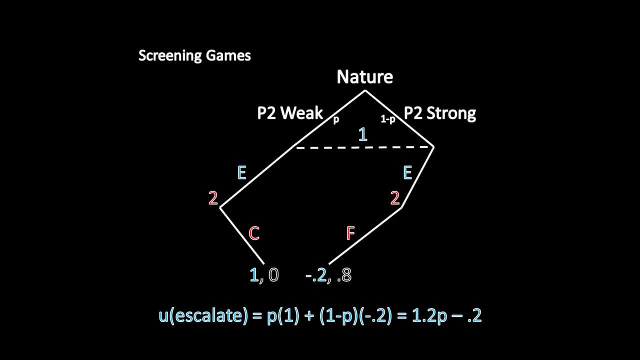 for escalation for player 1, which is going to be 1.2p minus 0.2.. If we want to figure out whether escalating is better than quitting, all we have to do is compare those two payoffs- And we're going to do that now- To figure out when escalating is better. 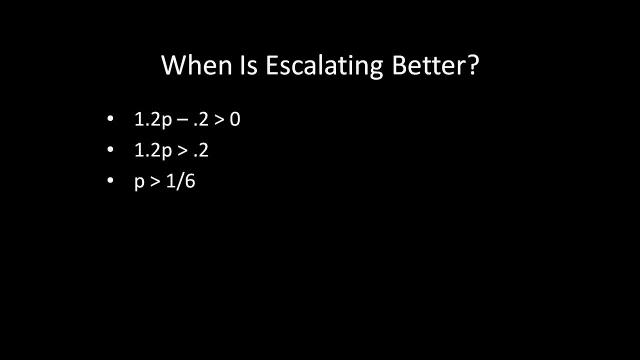 we need to take the utility for escalation and set that greater than the utility for quitting. That gives us 1.2p minus 0.2 greater than 0. Do a little bit of rearranging and solve for p and you get p greater than 1 sixth. So that is saying that if player 1's belief that player 2 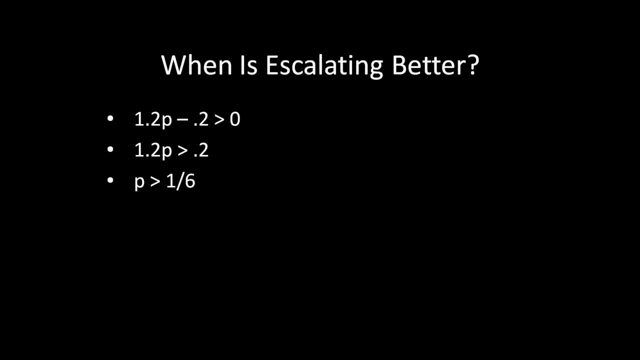 is weak is greater than 1 sixth, then player 1 prefers to escalate And analogously, if we flip that inequality, we figure out when player 1 prefers quitting, and obviously that's going to be when p is less than 1 sixth. 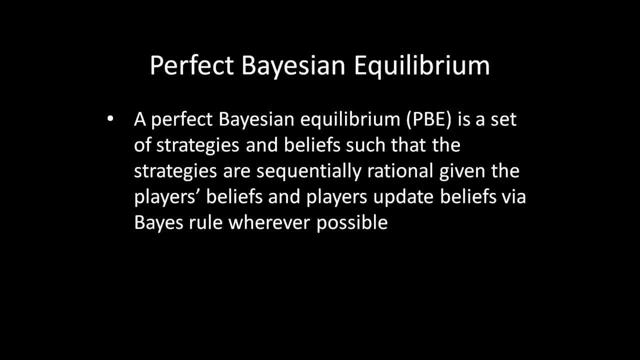 We can now put all of this together. If you remember, back to last time, this was our definition of perfect Bayesian equilibrium And, specifically, we need a set of strategies and beliefs. So we've figured out all of that. The beliefs part is actually straightforward. 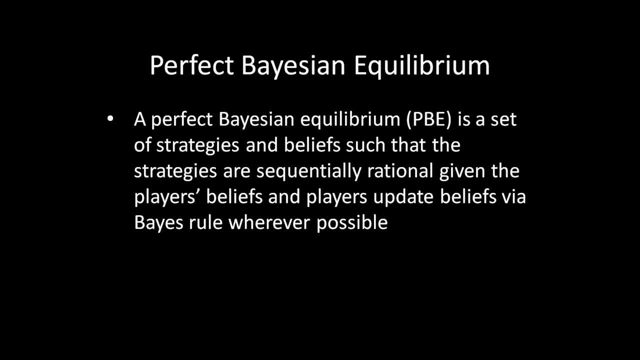 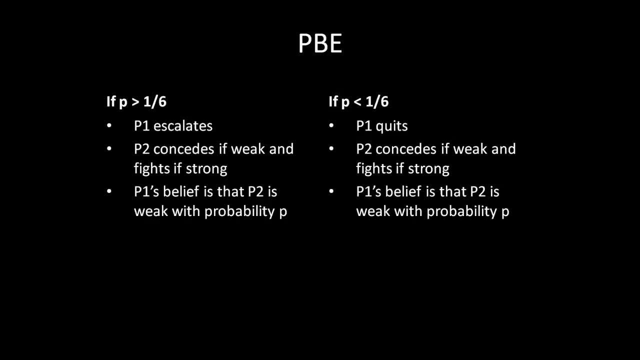 we don't have to do any sort of extra calculation for that, because there's no updating in this screening game. It's just a prior belief. So if we put everything together, the perfect Bayesian equilibrium is going to be a function of that prior belief. This is why we care so much about beliefs in Bayesian games. 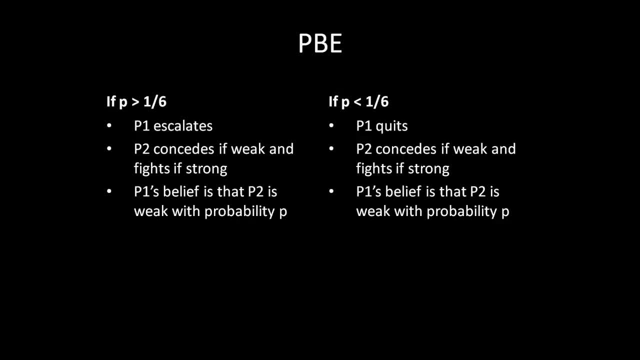 It's because it drives what happens in equilibrium. So if p is greater than 1, sixth, then player 1 is going to escalate and player 2 will concede if weak and fight if strong. So that takes care of the strategies. part of the perfect Bayesian. 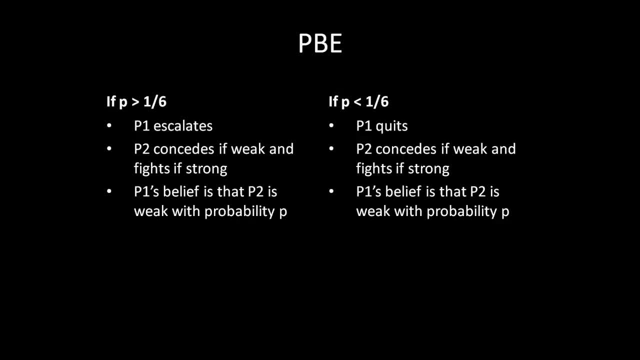 equilibrium. The remaining thing is to talk about that belief, But again, like I said, player 1 doesn't have to update his belief throughout the game. So player 1's belief is simply that player 2 is weak with probability p and nothing more. 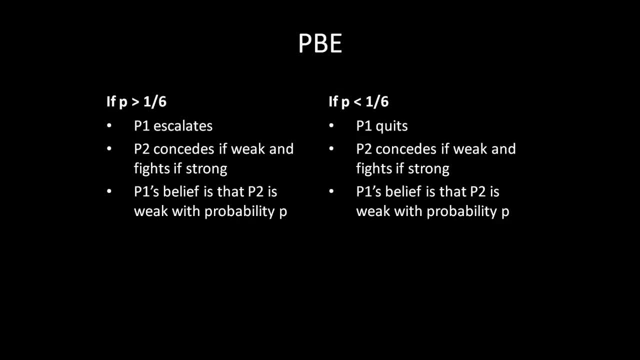 You'll also notice that we don't have a belief for player 2 here, and that's because player 2 has complete information, So there are no beliefs for player 2 to worry about. Meanwhile, if p is less than 1 sixth, then something different happens in equilibrium. 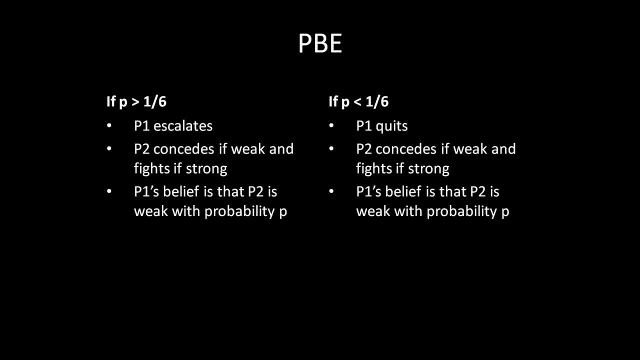 Player 1 quits and player 2 concedes if weak and fights if strong. So that part hasn't changed. Player 1's belief hasn't changed either — player 1's belief that player 2 is weak remains. probability p: 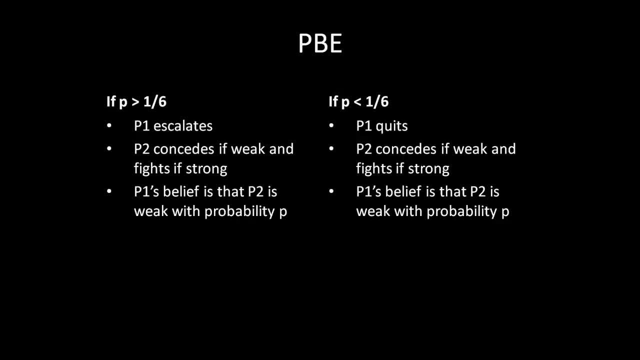 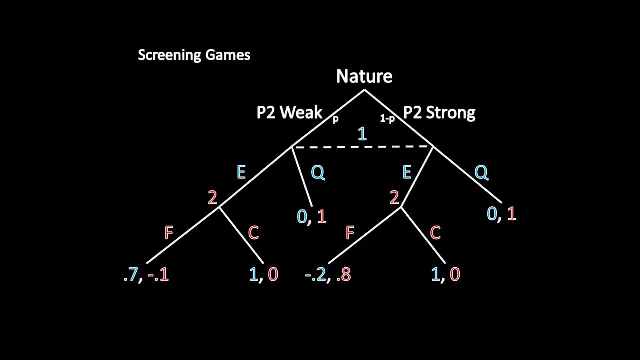 The last thing I want to talk about before we end today is why we call these things screening games. So if we go back to this game tree, what player 1 has the option of doing is escalating to screen-out types or quitting to not screen out types. 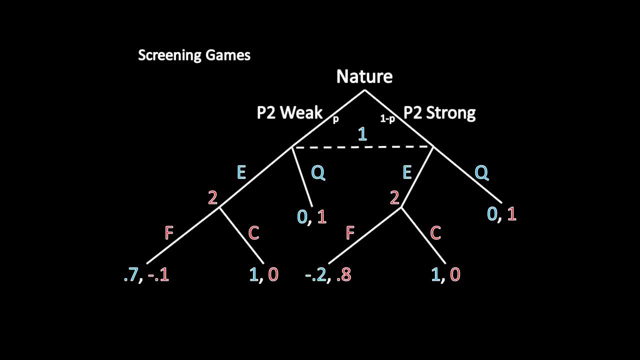 That is, if player 1 escalates, then the weak type is going to concede the issue and the strong type is going to fight. So it elicits different behavior out of Player 2. It screens or filters out one type to do one thing and forces the other type to do another thing. 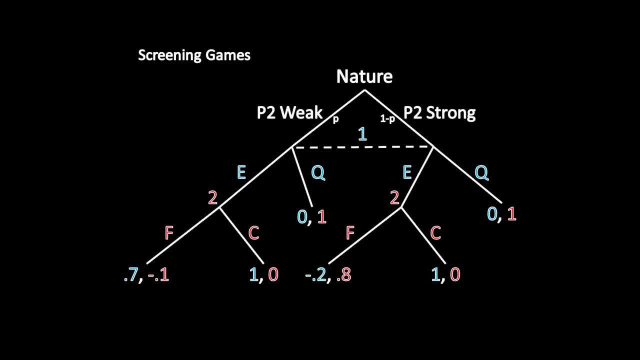 It may not be as apparent why we would still call this a screening game if Player 1 quits ahead of time, because if Player 1 quits then there's no screening behaviors following that, it's just the end of the game. But this would still be called a screening game because Player 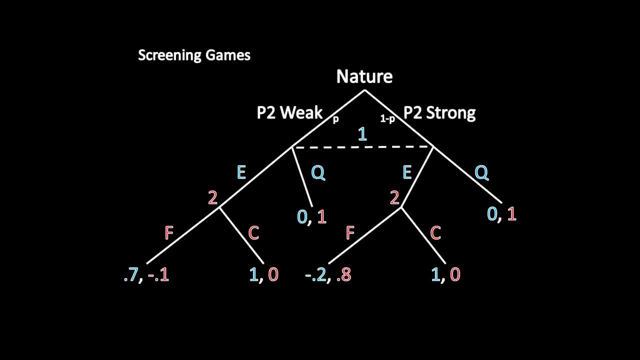 1 is declining the option to try to screen out Player 2's types. Alright, that wraps up this lecture on screening games. Hope you enjoyed it and hope to see you next time. Take care.